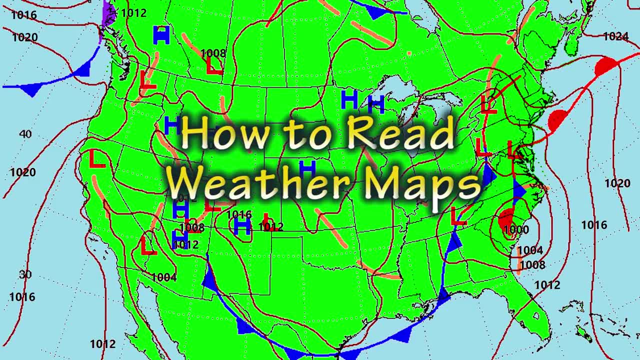 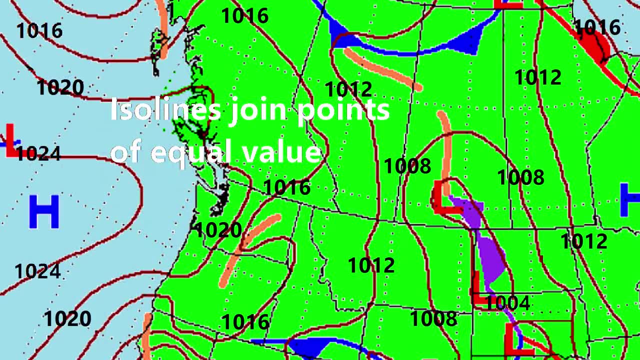 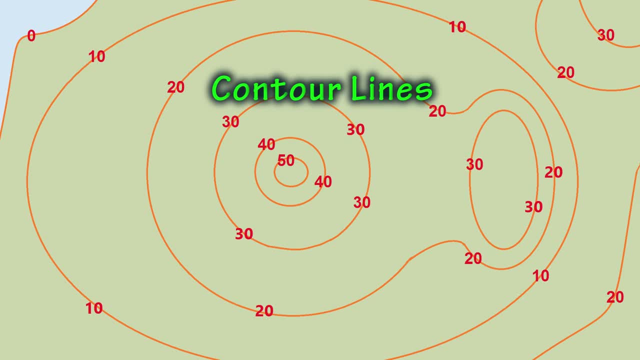 Weather maps, also known as the synoptic chart, are an example of an isoline map. Isoline maps are made up of lines that join points of equal value. Contour lines drawn on a topographic map are another example of an isoline map. 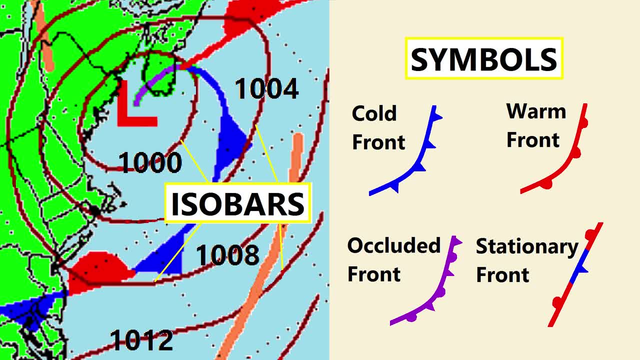 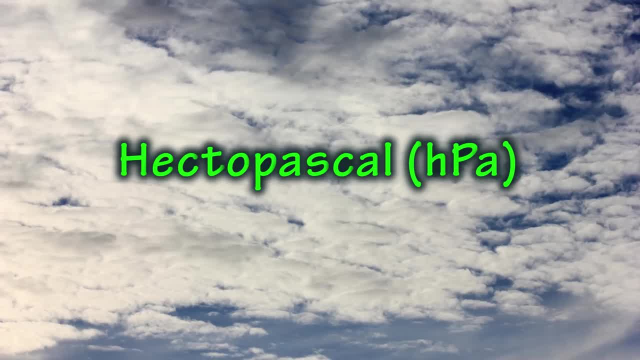 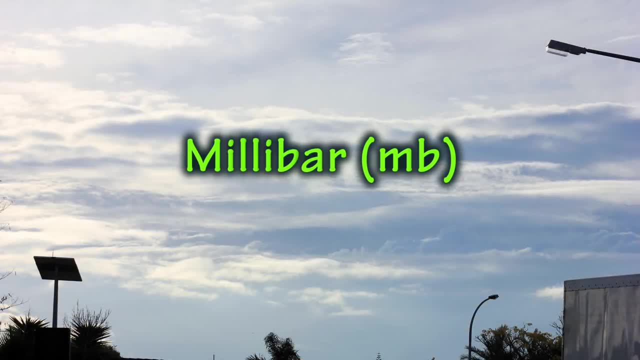 Weather maps use lines called isobars plus other symbols to join together lines of equal air pressure. Today most meteorologists use the hectopascal for measuring atmospheric pressure. Many weather reports to the public use the millibar. One hectopascal equals one millibar. 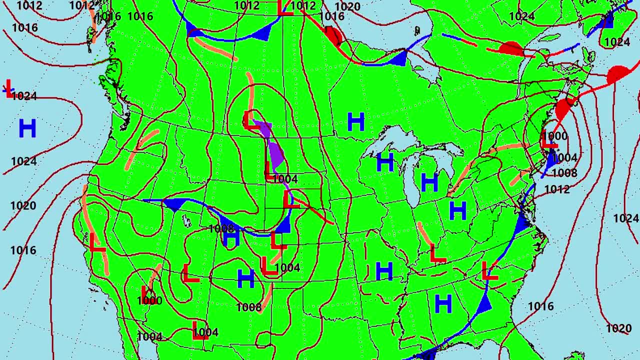 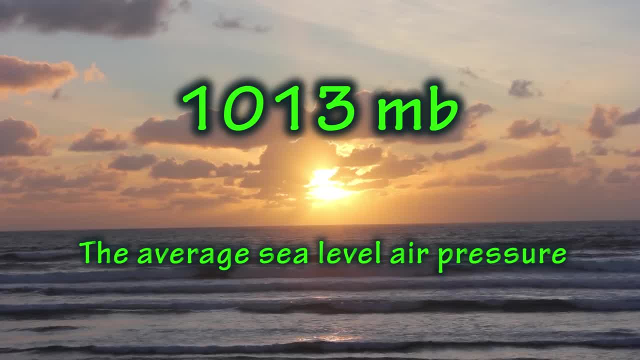 On these American weather maps, the isobars are drawn at intervals of four millibars. 1,013 millibars is the average sea level air pressure. Therefore, areas with an air pressure of 1,013 millibars are drawn at intervals of 4 millibars. 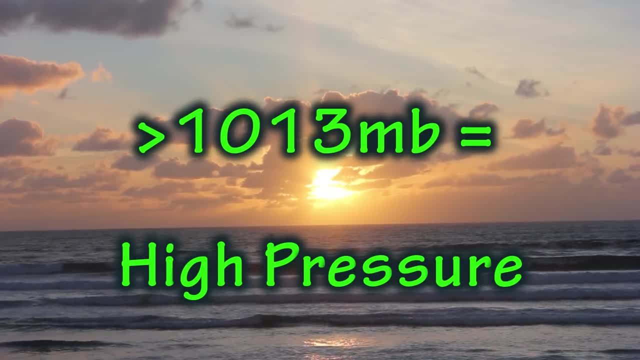 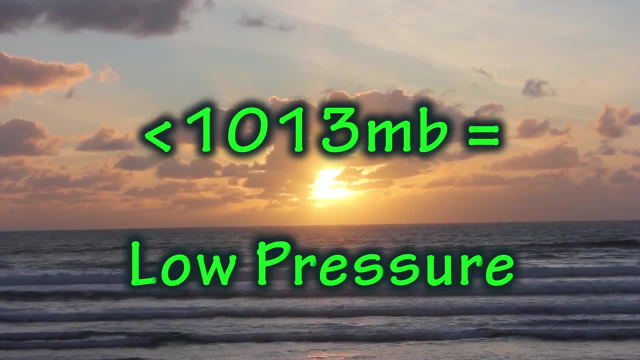 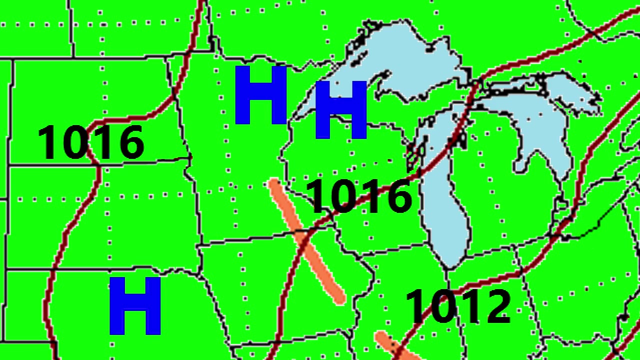 The areas with an air pressure of over 1,013 millibars are considered to be areas of high pressure, and areas with an air pressure below 1,013 millibars are considered to be areas of low pressure. On a weather map, areas of high pressure or anticyclones are identified by a letter H. 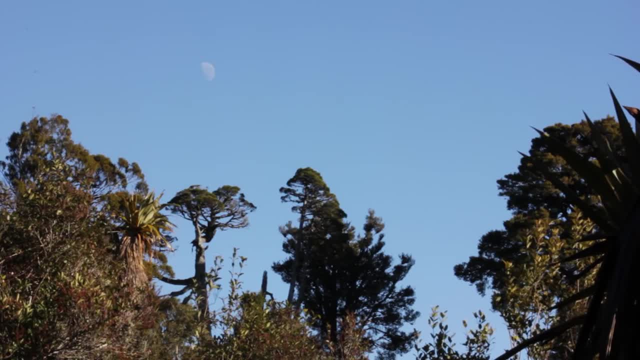 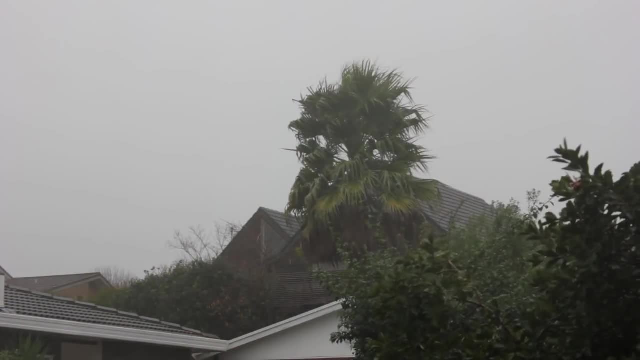 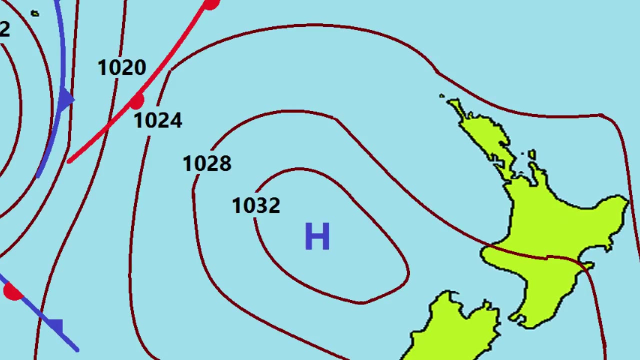 These areas are associated with clear skies and little wind. Areas of low pressure or depressions are usually identified by a letter H And are associated with rain, clouds and high winds. High pressure systems have enclosed isobars which increase in pressure towards their centre. 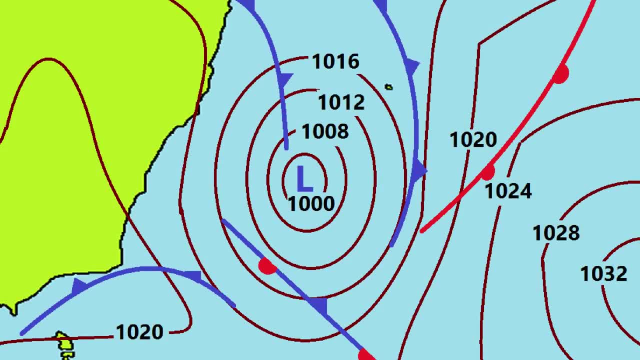 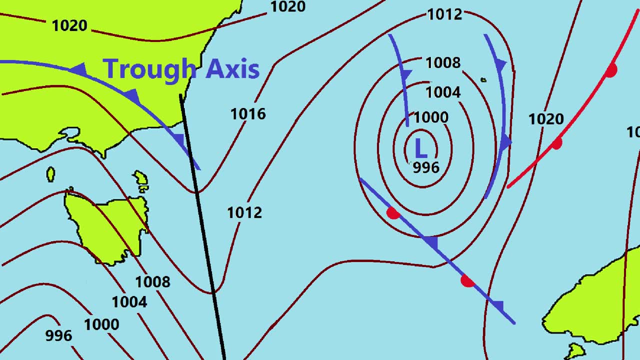 Low pressure systems, on the other hand, contain isobars which decrease in pressure towards the centre. When isobars make a sharp bend around a low, this bend area is called a trough. One of the main symbols employed on a weather map is called veneer. 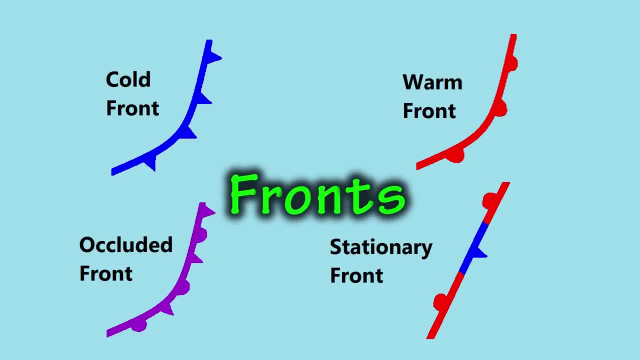 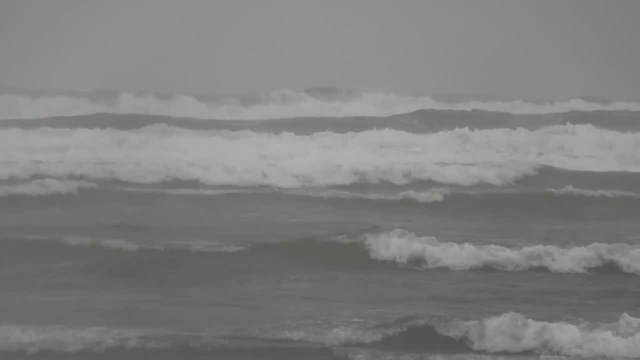 The front represents the boundary between two air masses and appears on the weather map as a line with triangles or semicircles attached. At the front of two air masses there is stormy weather. There are four types of front most commonly seen on weather maps: 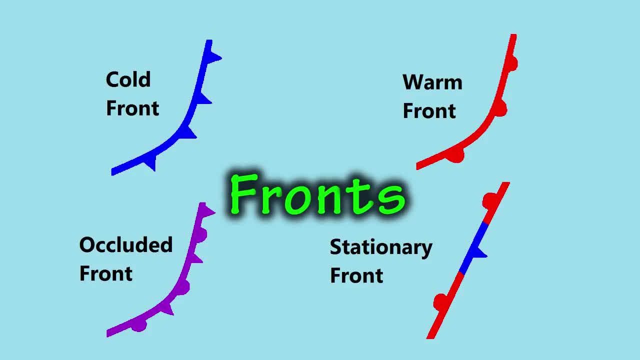 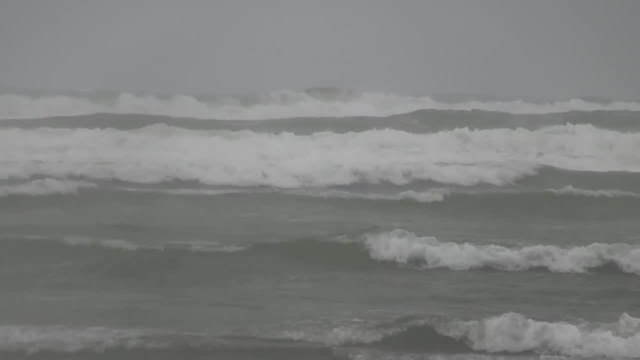 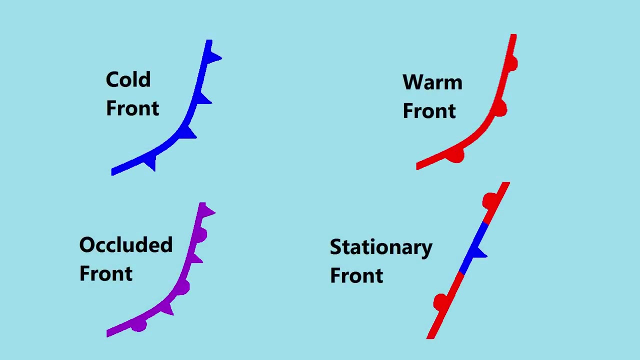 A front represents the boundary between two air masses and appears on the weather map as a line with triangles or semi circles attached. At the front of two air masses there is stormy weather. There are four types of front most commonly seen on weather maps: 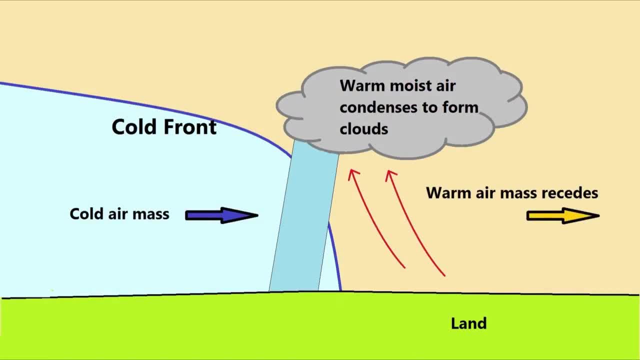 A cold front is the boundary where a cold air mass pushes underneath a warm air mass, forcing the warm air mass upwards, which forms clouds and rain. A cold front is the boundary where a cold air mass pushes underneath a warm air mass, forcing the warm air mass upwards, which forms clouds and rain. A cold front is for snow films- chop some heat, or for dust and multi-layered켜vers Very fine weather. weather is about twenty two degrees C, For snow occurs betweenén summer temperatures and Christmas a spectrum year conditions will be instead of two hours. 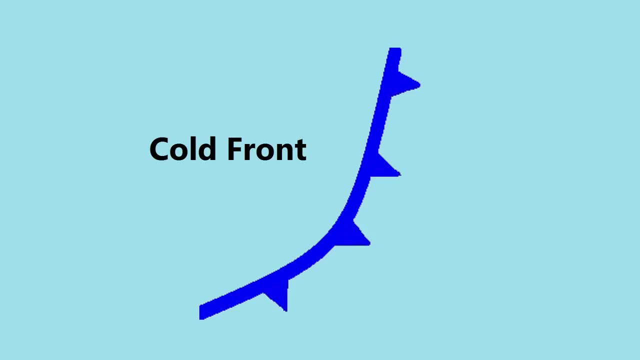 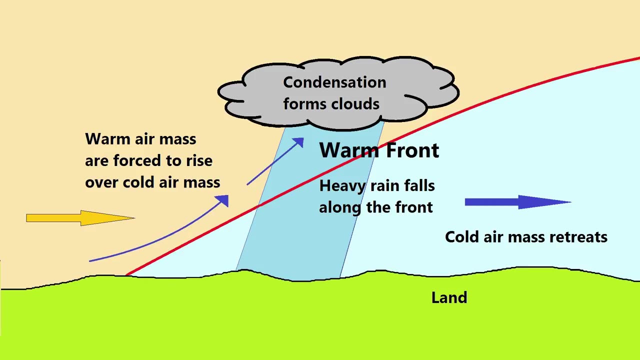 is represented by a blue line with the triangles pointing towards the direction of movement. A warm front is the boundary where a moving warm air mass is replacing a cold air mass. A warm front is represented as a red line with semi-circles pointing towards the direction of. 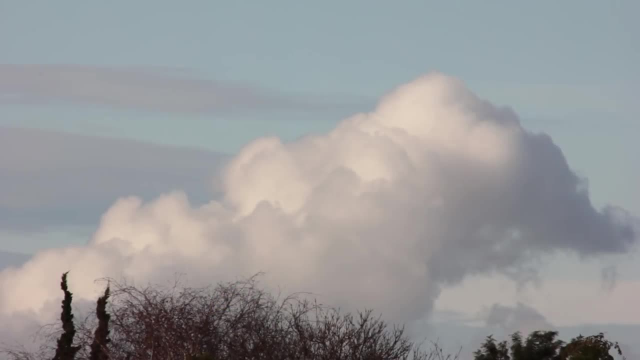 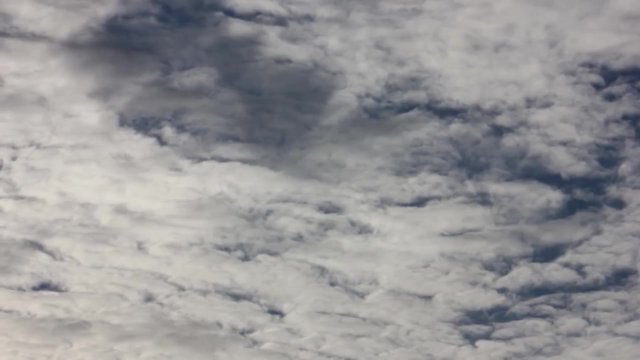 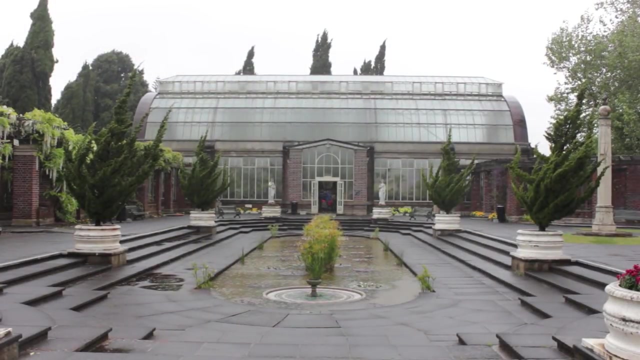 movement. Warm fronts move more slowly than cold fronts because it is harder for warm air to push against the denser cold air. As the warm air rises above the cold air, water vapor condenses, forming high clouds. Light precipitation can fall on areas as the warm front passes. A stationary 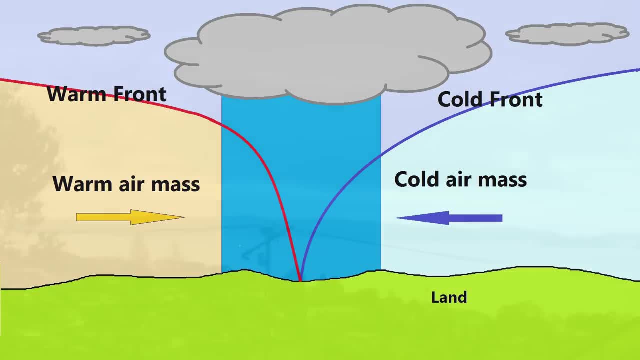 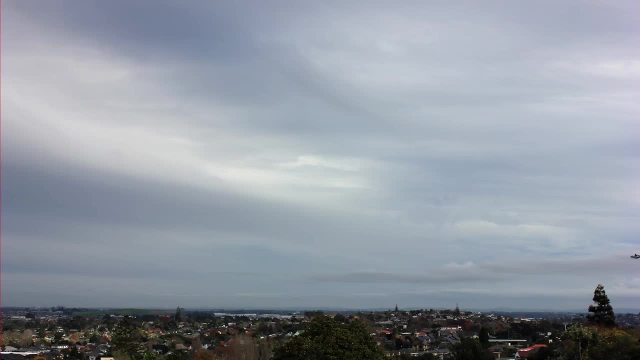 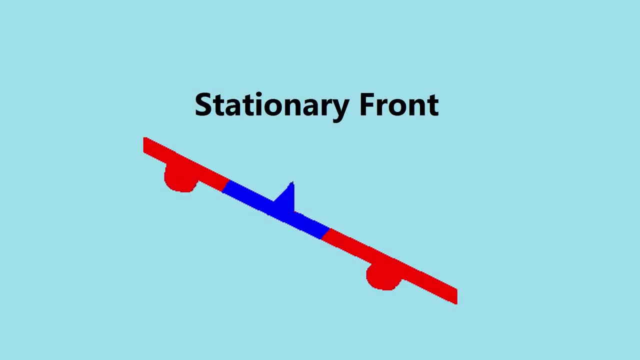 front is the boundary between two air masses which are not moving. Neither mass is strong enough to move the other. therefore, a stationary front can be pushing back and forth over a given area for days. A stationary front is represented as alternating warm and cold front symbols. 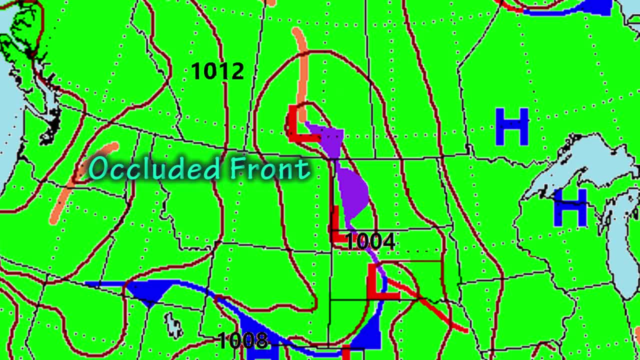 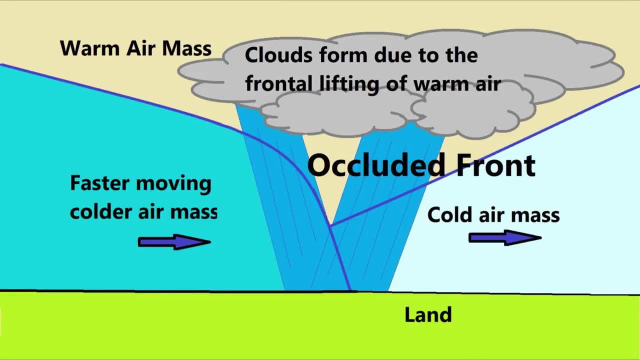 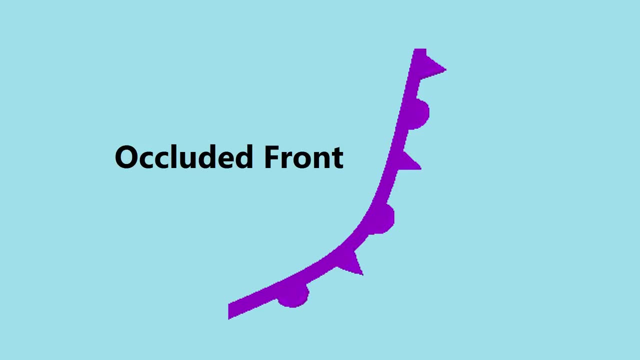 An occluded front is a composite of two frontal systems that merge. as a result of occlusion. Cold fronts generally move faster than warm fronts. therefore, the cold front will overtake a warm front and force it aloft. An occluded front is represented as a purple line with triangles and. 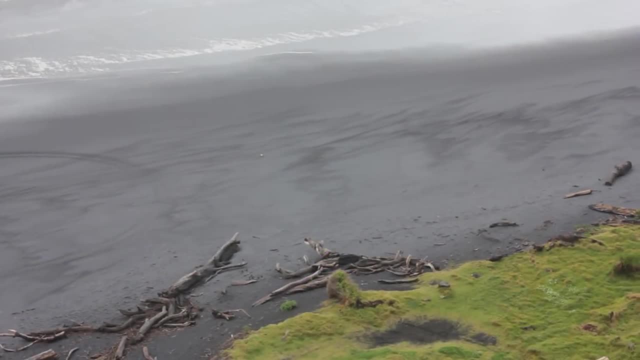 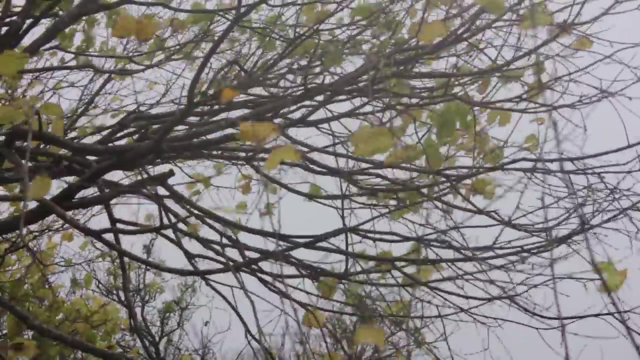 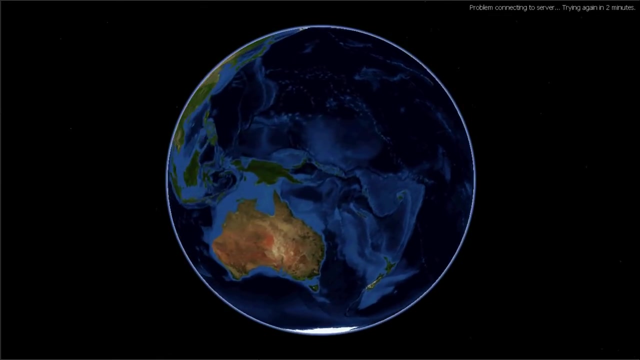 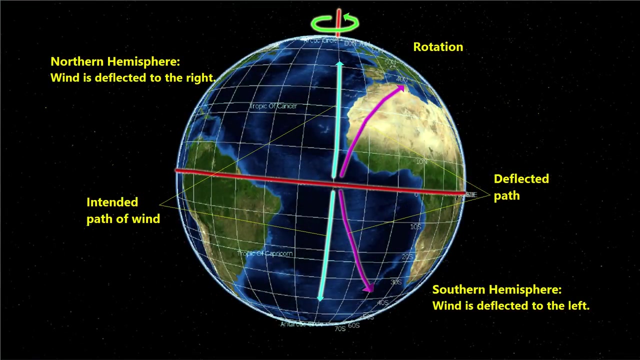 semi-circles Weather maps also show wind conditions. Wind is the movement of air. Wind moves from high to low pressure areas. Winds do not travel in a straight line due to the Coriolis effect. This effect is created by the rotation of the earth. The Coriolis effect deflects wind to the 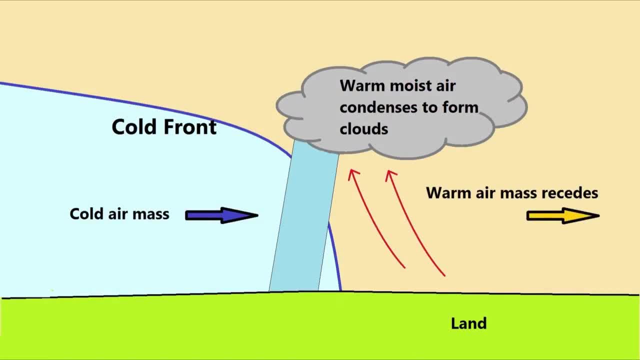 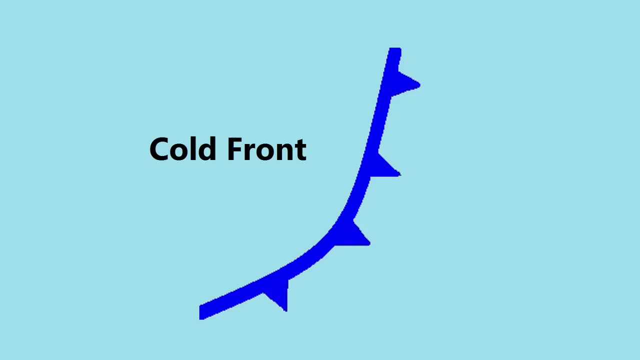 A cold front is the boundary where a cold air mass pushes underneath a warm air mass, forcing the warm air mass upwards, which forms clouds and rain. A cold front is the boundary where a cold air mass pushes underneath a warm air mass, which forms clouds and rain. 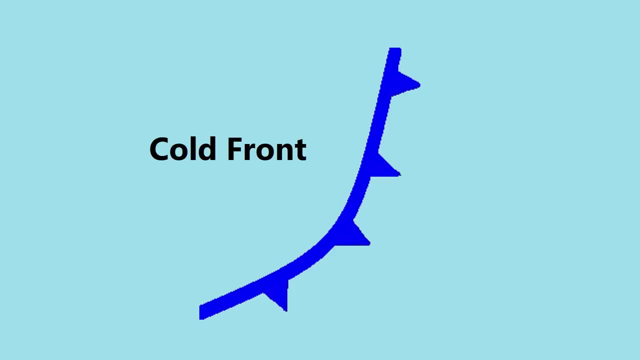 A cold front is represented by a blue line with the triangles pointing towards the direction of movement. A warm front is the boundary where a moving warm air mass is replacing a cold air mass. A warm front is represented as a red line with semicircles pointing towards the direction of movement. 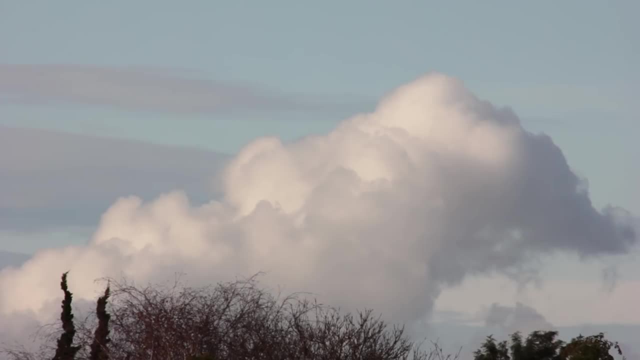 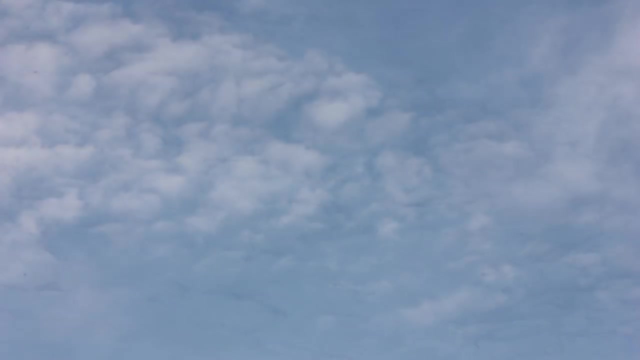 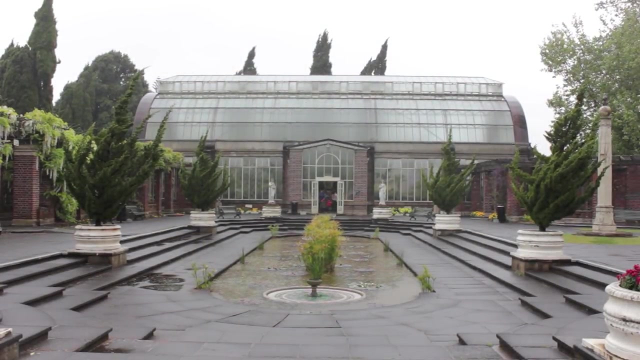 Warm fronts move more slowly than cold fronts because it is harder for warm air to push against the denser cold air. As the warm air rises above the cold air, water vapour condenses, forming high clouds. Light precipitation can fall on areas as the warm front passes. 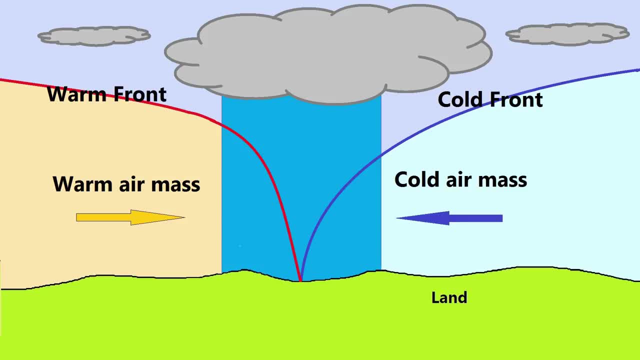 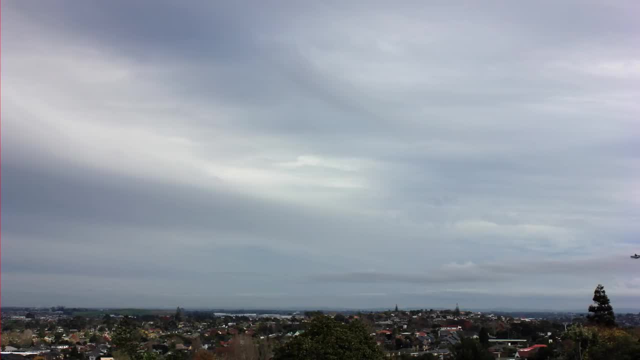 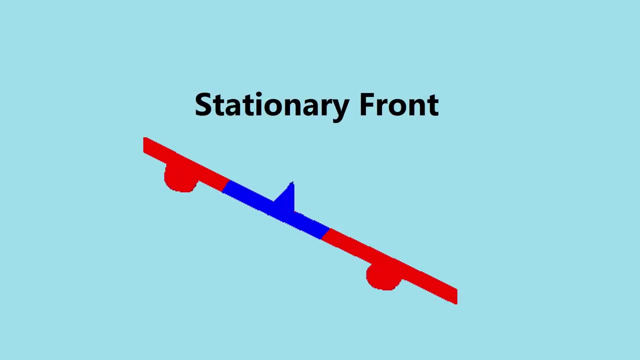 A stationary front is the boundary between two air masses which are not moving. Neither mass is strong enough to move the other. therefore, a stationary front can be pushing back and forth over a given area for days. A stationary front is represented as an alternating warm and cold front symbols. 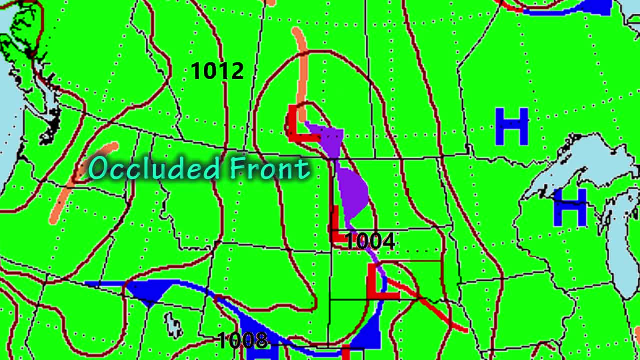 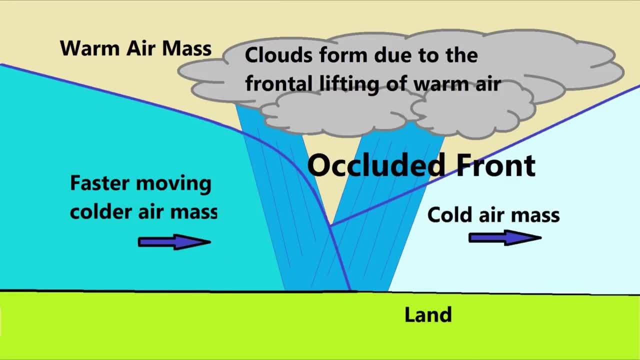 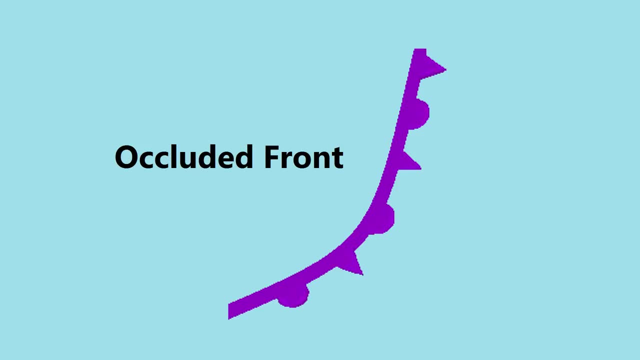 An occluded front is a composite of two frontal systems that merge. as a result of occlusion, Cold fronts generally move faster than warm fronts. therefore, the cold front will overtake a warm front and force it aloft. An occluded front is represented as a purple line with triangles and semicircles. 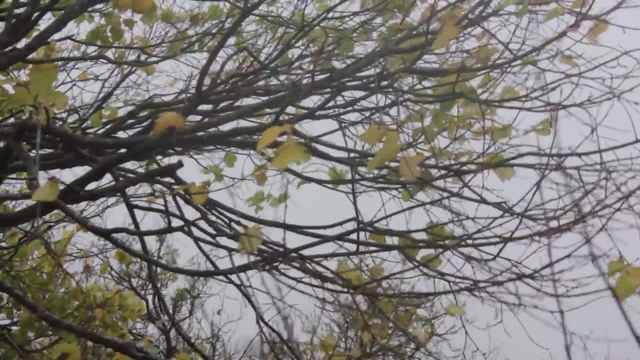 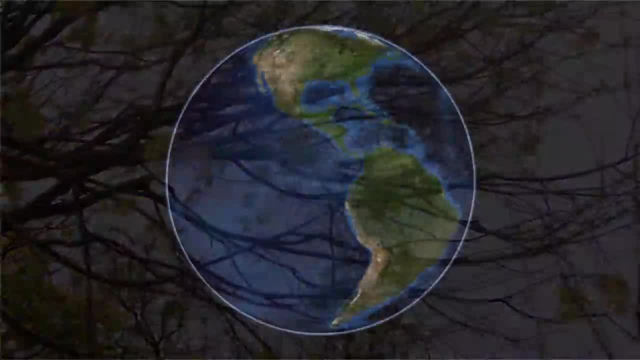 Weather maps also show wind conditions. Wind is the movement of air. Wind moves from high pressure areas towards low pressure areas. Wind moves from high pressure areas to low pressure areas. Winds do not travel in a straight line due to the Coriolis effect. 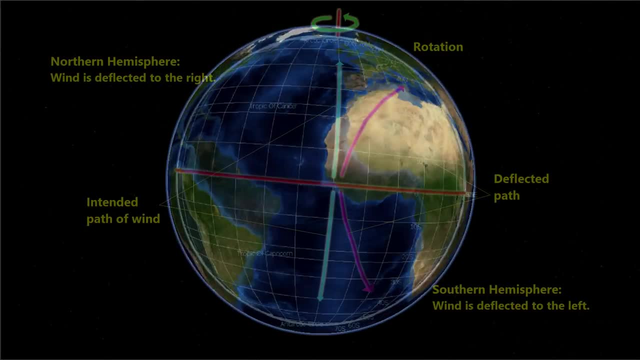 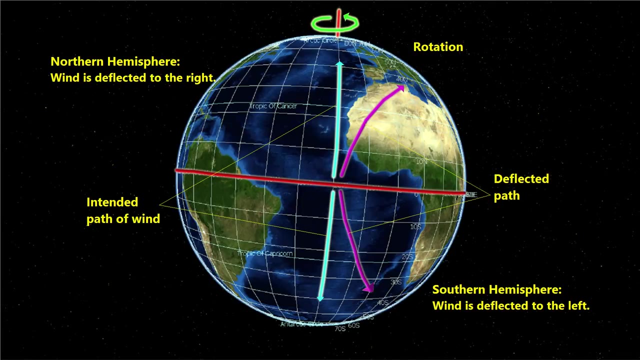 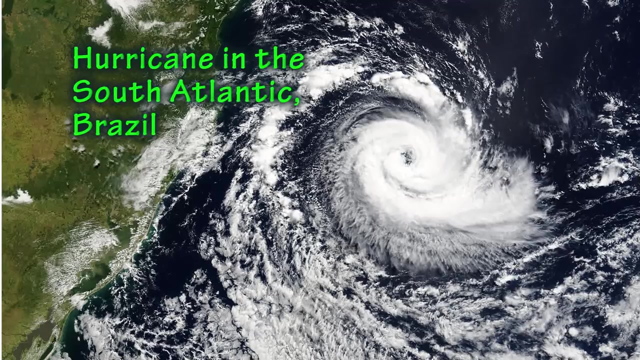 This effect is created by the rotation of the earth. The Coriolis effect deflects wind to the left in the southern hemisphere and to the right in the northern hemisphere. Thus, in the southern hemisphere wind flows clockwise around low pressure systems and anti-clockwise in high pressure systems. In the northern hemisphere: wind flows anti-clockwise around low pressure systems. In the northern hemisphere, wind flows anti-clockwise around high pressure systems. In the northern hemisphere, wind flows anti-clockwise around low pressure systems. In the northern hemisphere, wind flows anti-clockwise around high pressure systems. 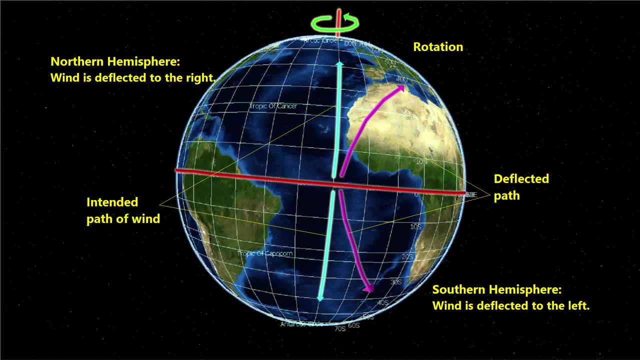 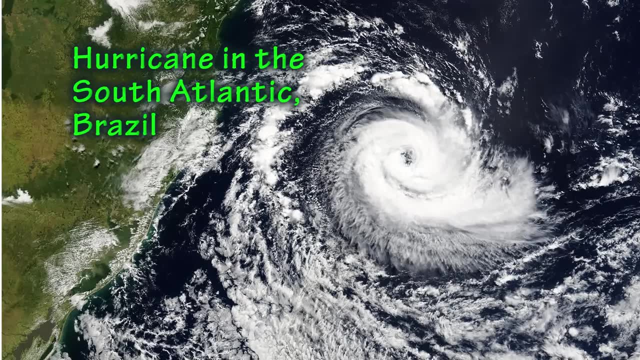 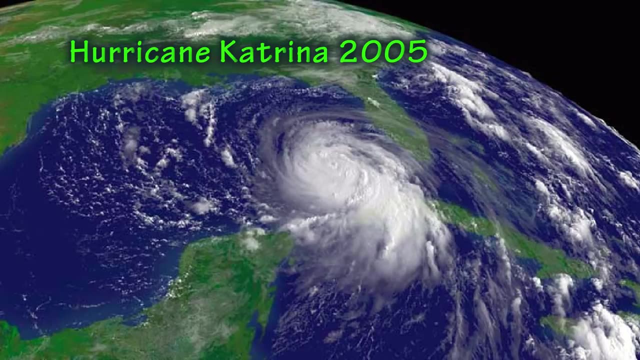 left in the southern hemisphere and to the right in the northern hemisphere. Thus, in the southern hemisphere wind flows clockwise around low pressure systems and anti-clockwise in high pressure systems. In the northern hemisphere, wind flows clockwise around low pressure systems and clockwise around high pressure systems. 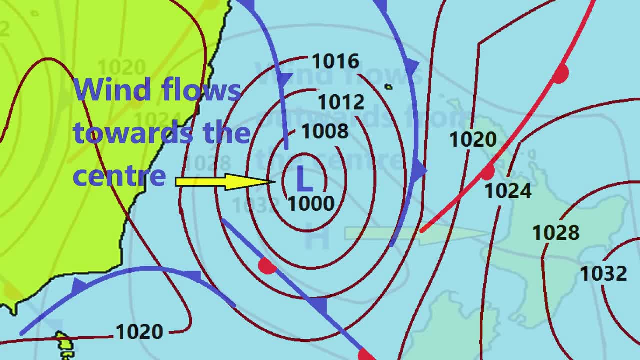 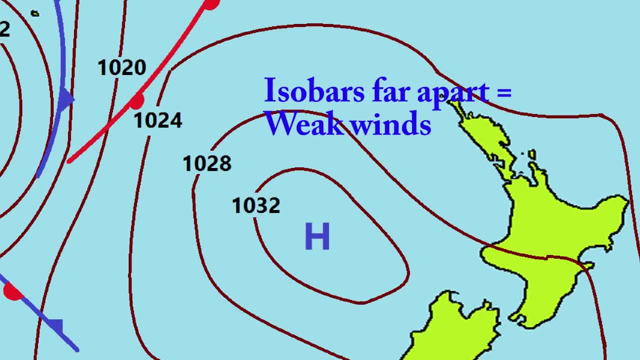 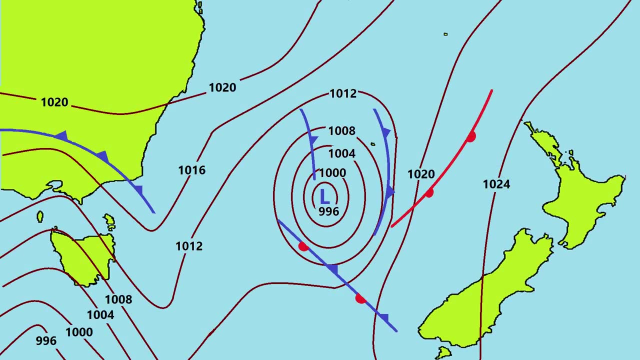 Generally, wind flows towards the centre of low pressure systems and away from high pressure systems. When isobars are close together, wind is strong. When isobars are far apart, wind is weak. Now it is time for you to go and read some weather maps and see if you can interpret them. 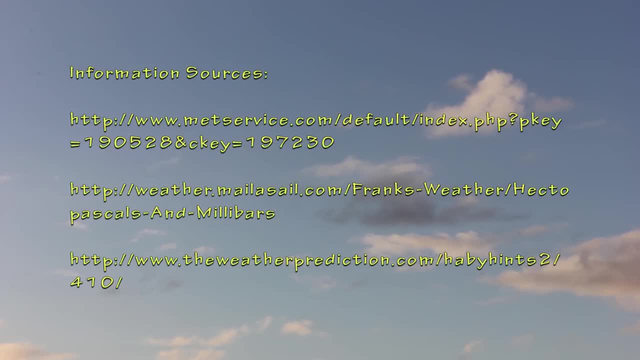 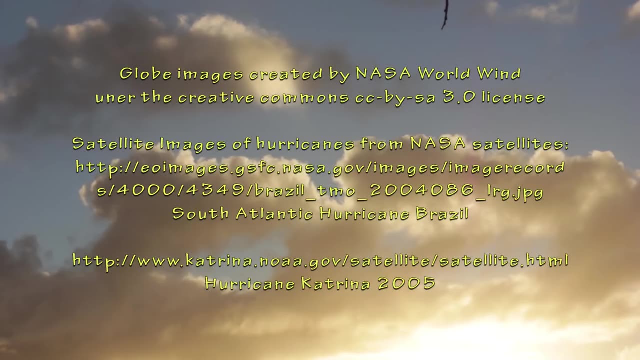 If you have any questions or other problems, please post them in the comments section below. Thank you for watching this video. If you have any questions or other problems, please post them in the comments section below. Thank you. 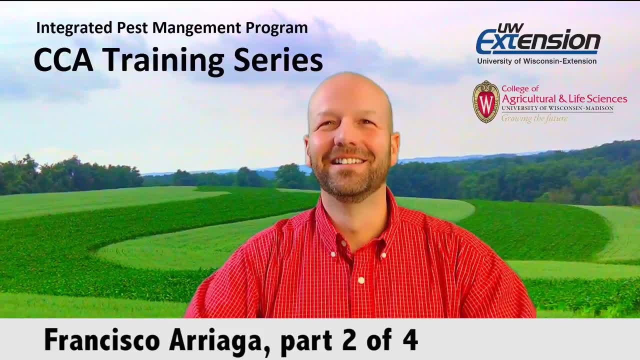 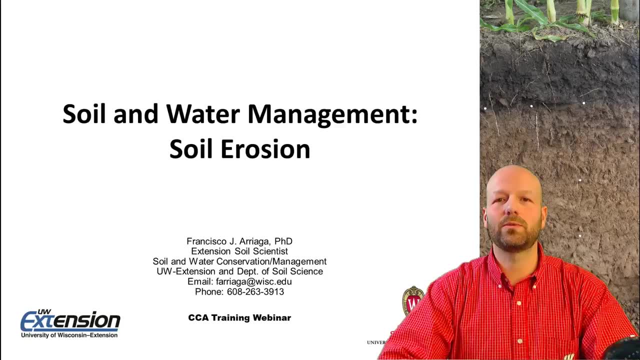 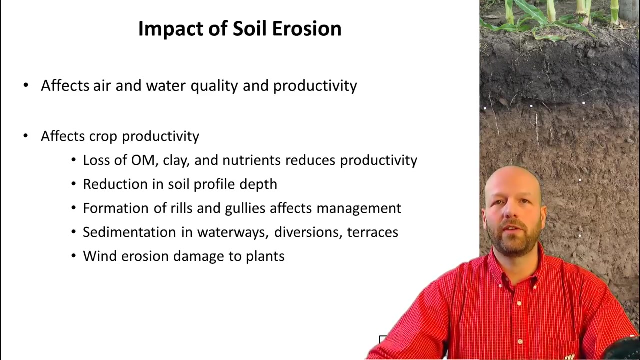 Hi, my name is Francisco Arriaga. I'm a soil science extension specialist with the University of Wisconsin-Madison And I'll be discussing now another topic on soil and water management: soil erosion. So let's get into it. So we know that erosion- soil erosion- impacts many different things, but we know it affects air and water quality and, obviously, productivity. 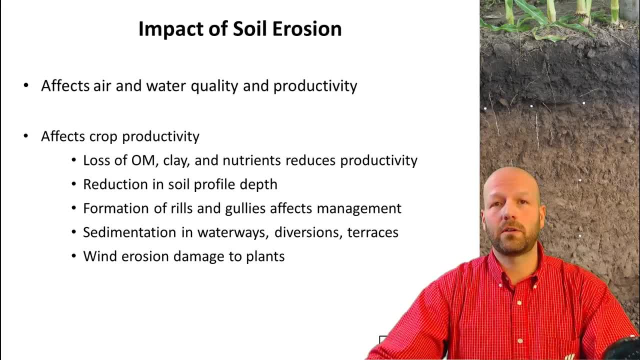 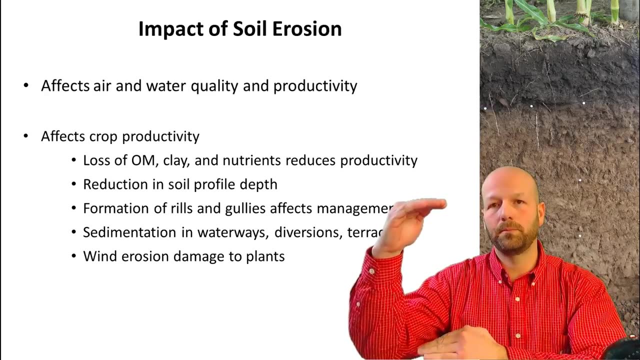 And so these effects on productivity are related a lot of times to the loss of organic matter nutrients and reduction of productivity from those. But also the other thing that happens long term is that the depth of the soil profile- so the depth of soil that roots have to explore it- decreases because you're removing the surface soil.